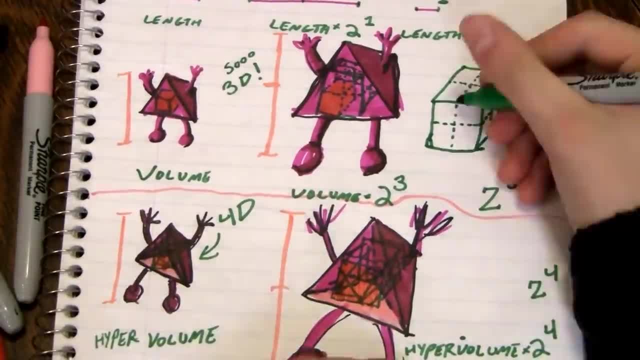 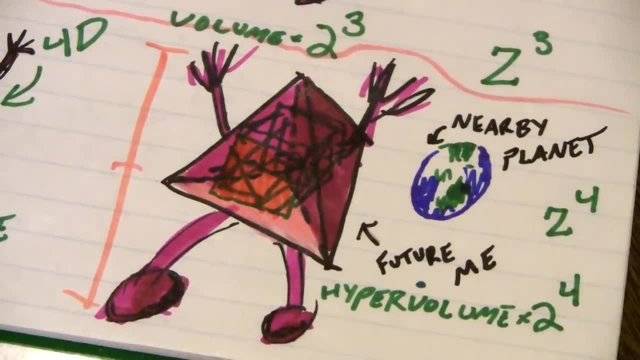 it's that amount to the n. So when you put it like that, you're actually making pretty good use of your limited time on this earth, And by limited time on this earth I mean that we're all going to become immortal space robots. Anyway, you're continuing your plans for a 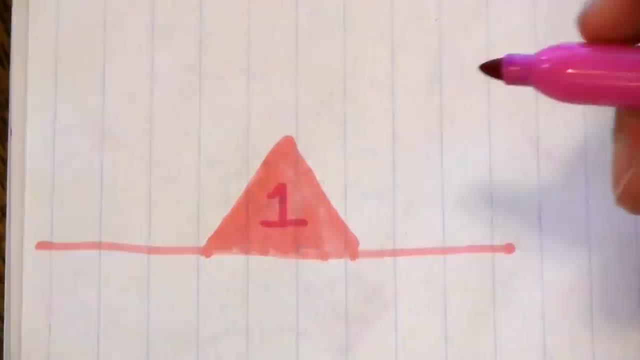 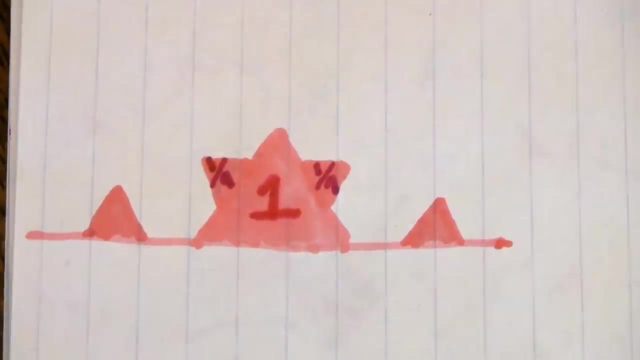 fractal city of infinite dragon dungeons. Triangles upon triangles upon triangles, each next set scaled down by a factor of three, That's one-ninth the area, but there's four times as many, And the next set has four times as many. 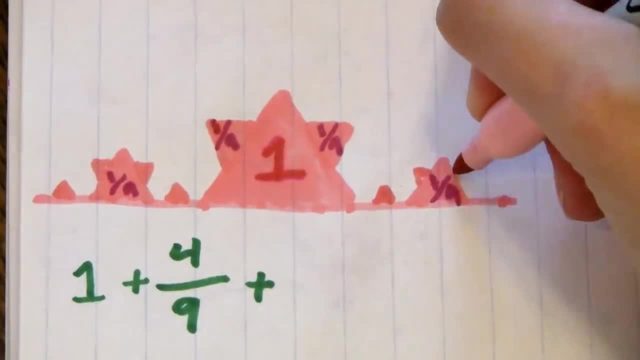 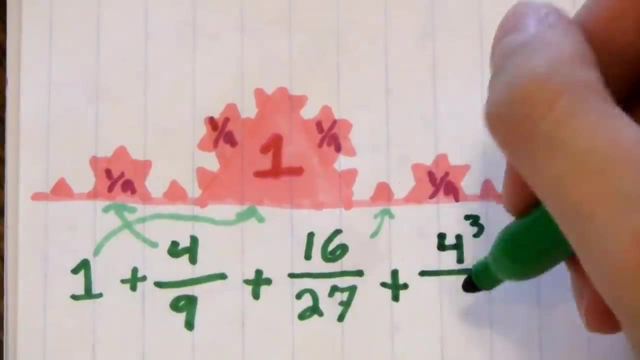 as the last, but one-ninth times the size of the last. So the total weight of steel is one plus four-ninths plus four, squared over nine, squared plus four to the three, over nine to the three. dot, dot, dot, plus four to the n over nine to the n, And maybe you could learn how to add up an. 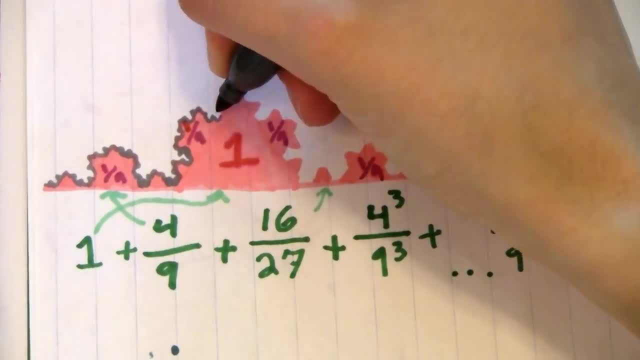 infinite series of numbers, if your teacher would ever get past logarithms. but at least you know how to create the perfect fractal city, which is good, because understanding scale factors and city planning seems like a lot of work. So let's get started. 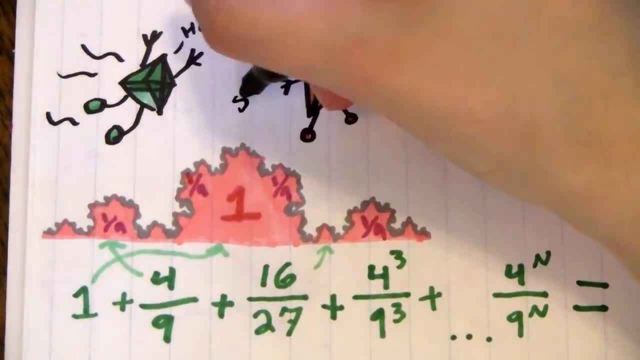 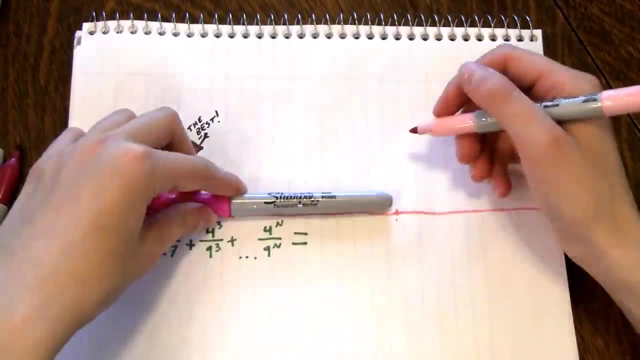 So let's get started. the kind of thing that might come in handy if you want to help the species on our journey towards becoming immortal space robots. Really, the only thing that could make the city better is if it were twice as big, Or how about three times as big, so you can keep this part of the 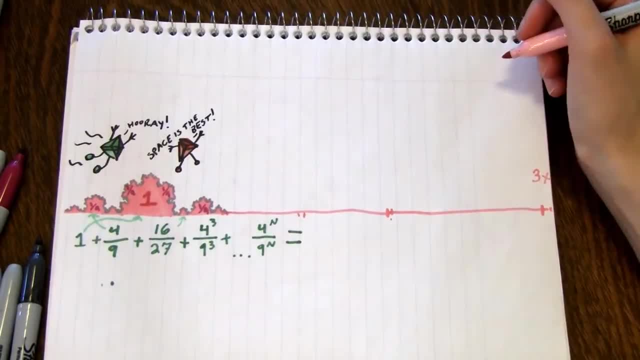 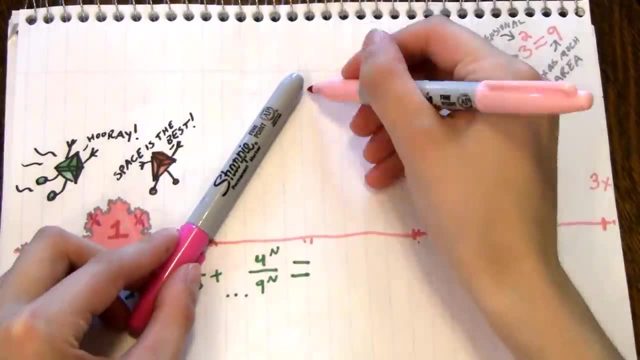 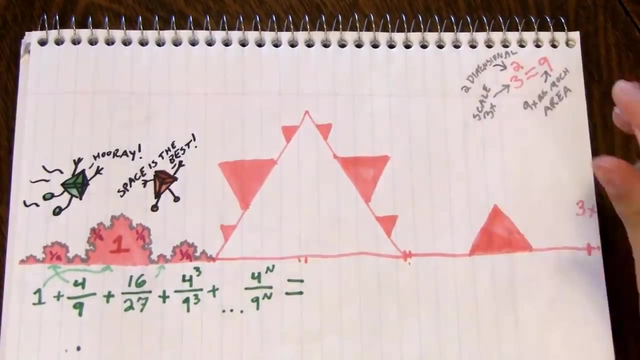 design and just draw the next iteration. Three times the scale in two dimensions means, technically you'll need nine times as much steel. though, as far as drawing these plans go, it's not nine times as difficult, but only four, since the hard part is the outside spiky part And that's just copied. 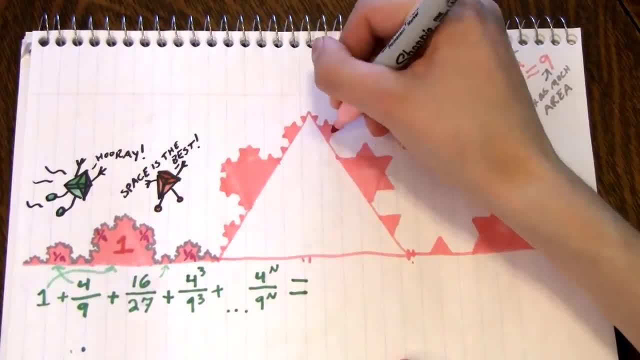 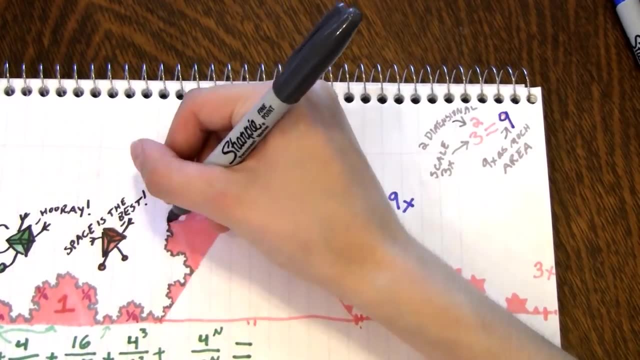 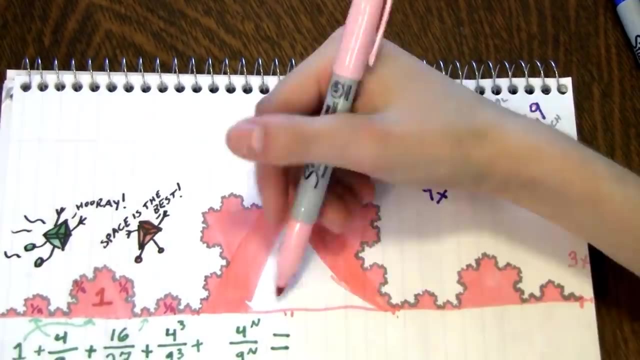 four times in order to scale up by three. Okay, wait, Weird thing number one: Scaling up by three makes nine times as much steel, but it's the same thing copied four times plus filling in this middle triangle, so it's also four times the steel plus nine. So if this mystery sum of an 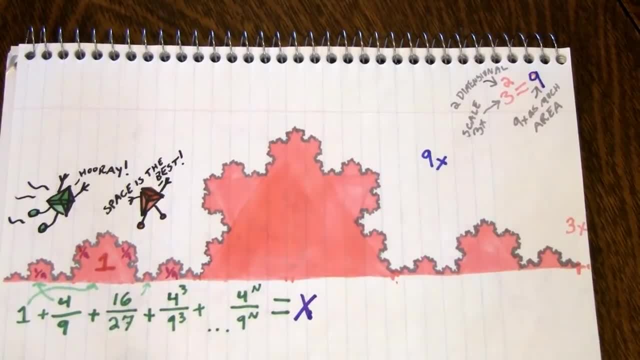 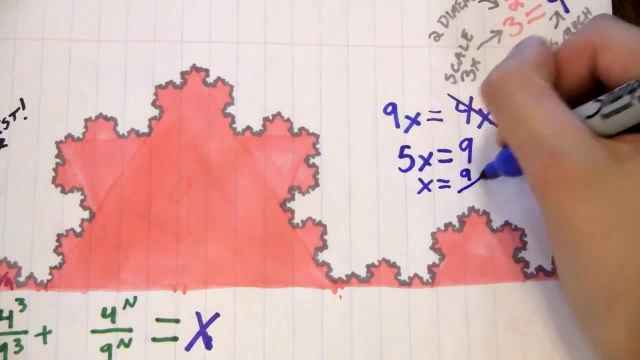 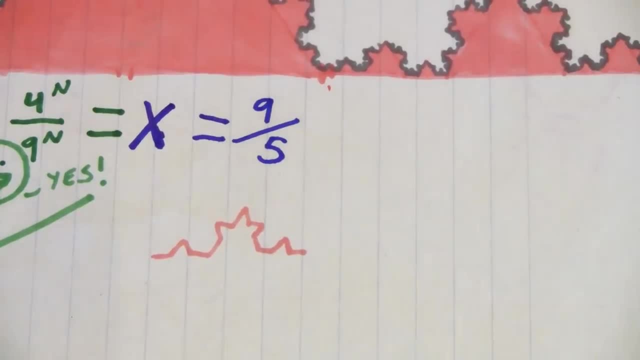 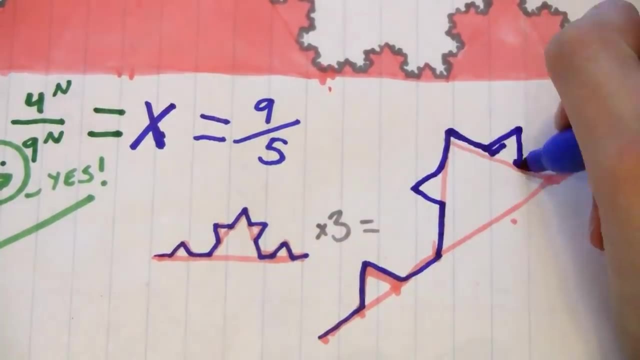 edge, the actual Koch curve not filled in. if it were a regular line, not an infinitely spiked one, scaling up by three would make it three times as much drawing as expected. but if that spiky line were supposed to represent an, 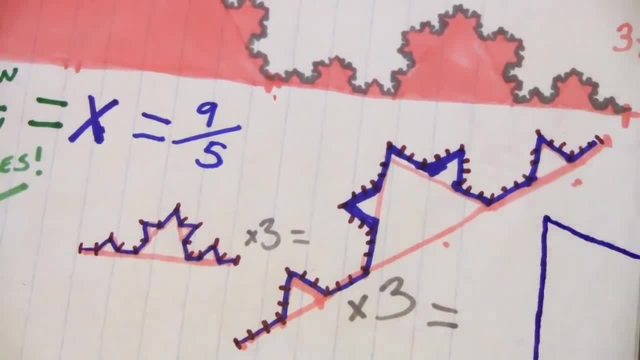 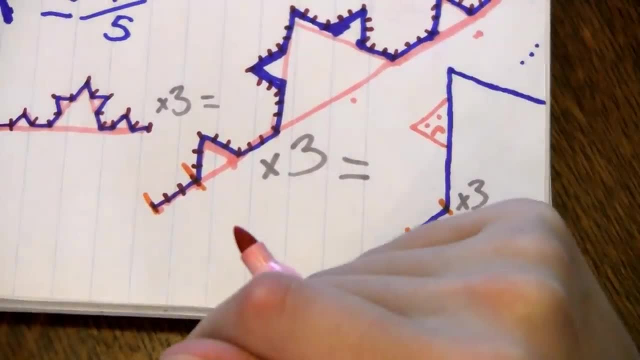 infinitely spiked magical fortress city of dragon dungeon doom. by scaling it up in this way, you'd be losing details, making these long lines that should have had spiky bumps in them. theoretically, no matter how much you scale up the city or no matter how finely you look at it, you'll never get any flat sections. this. 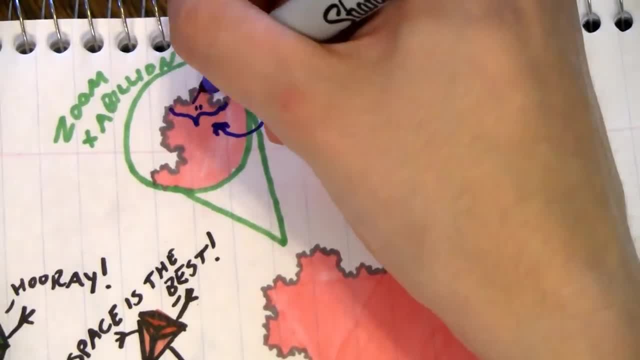 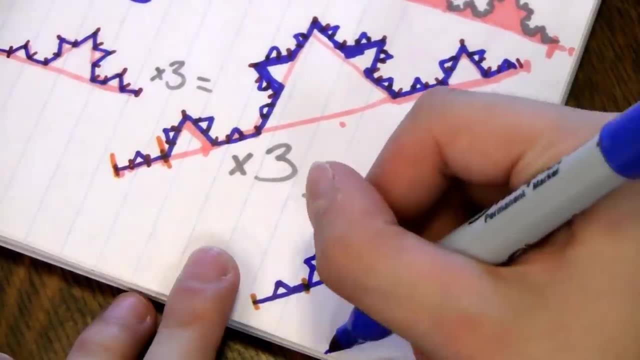 whole thing scaled down, is the same as this section, which is the same as this section, which is the same as this, and so on. three times as big is four times as much stuff, not three like if it were a normal 1d line, and certainly not nine. 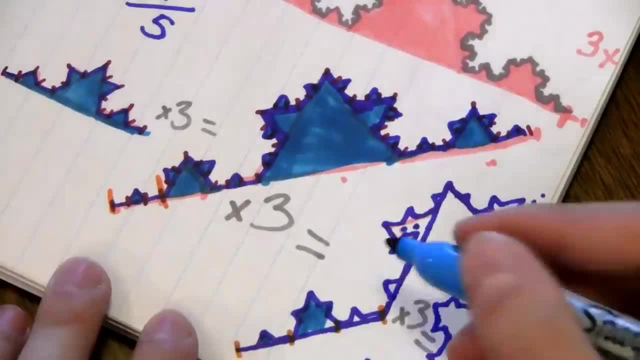 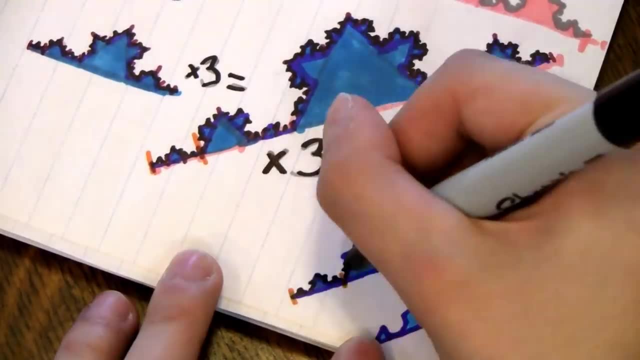 like the 2d area on the inside. somehow the infinity fractalness of the thing makes it behave differently from all 1d things and all 2d things. you convinced yourself that all 1d things got twice as big when you make them twice as big because you could think of them as 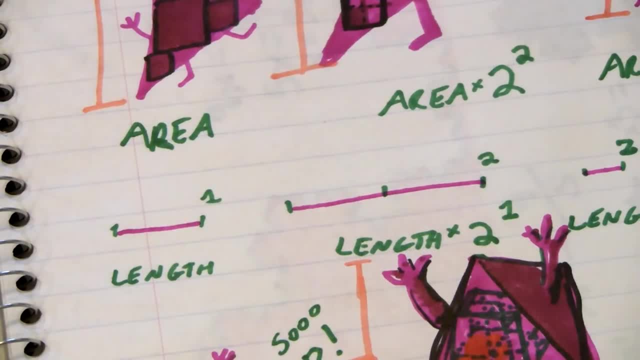 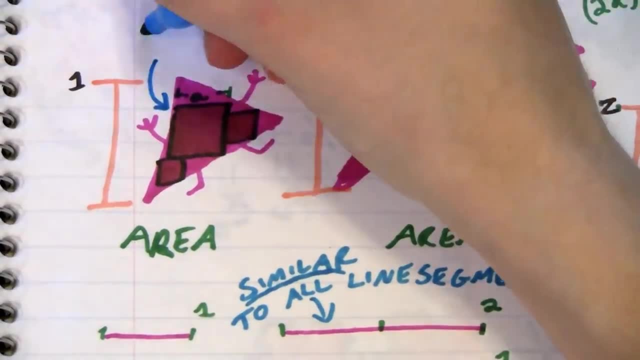 broken up into straight line segments and you know how line segments behave and you convince yourself: all 2d things scaled up by two get four times as much stuff, because 2d things can be thought of as being made of squares, and you know. 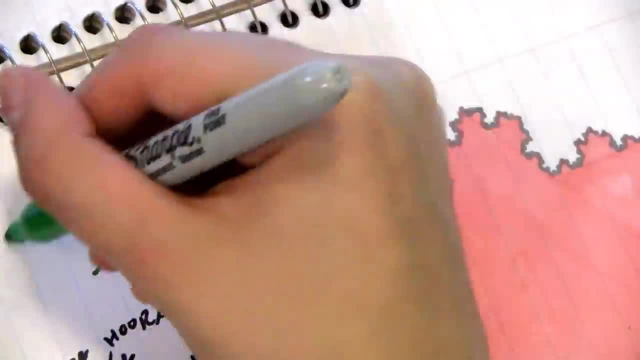 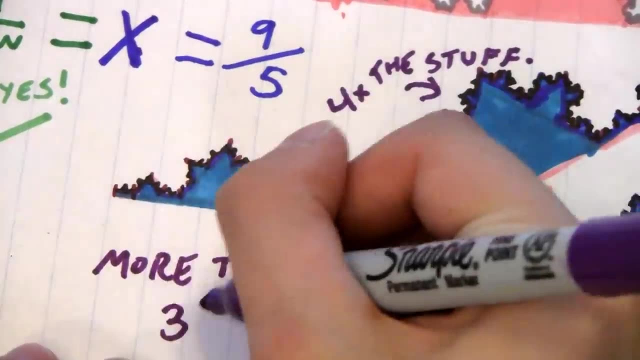 how squares behave. but then there's this, which has no straight lines in it and there's no square areas in it either: more than three to the one, less than three to the two. it behaves as if it's between one and two dimensions. 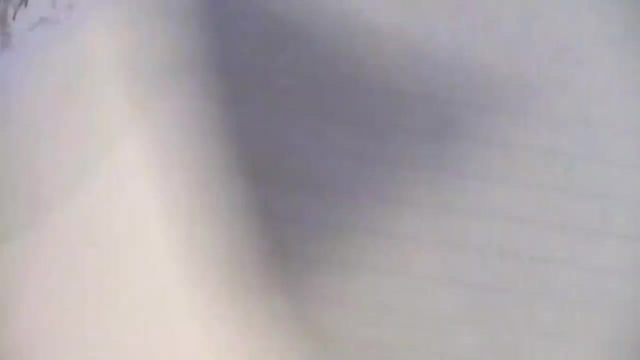 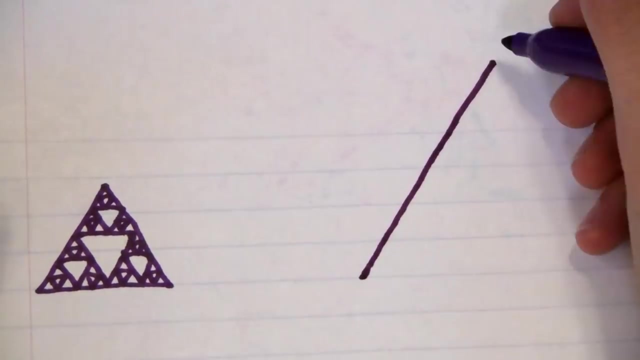 You think back to Sierpinski's triangle. Maybe it can be thought of as being made out of straight line segments, though there's an infinite amount of them and they get infinitely small When you make it twice as tall. if you just make all the lines of this drawing twice as 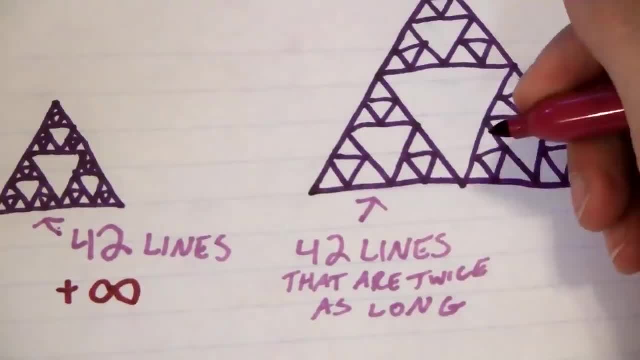 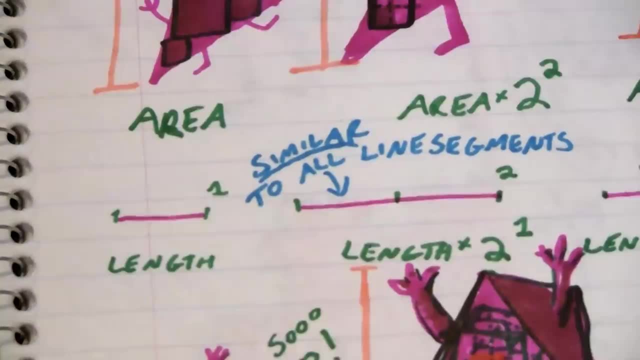 long. you're missing detail again. but the tiny lines too small to draw are also twice as long and now visible, and so on all the way down to the infinitely small line segments. Hmm, You wonder if your similar line thing works on lines that don't actually have length. 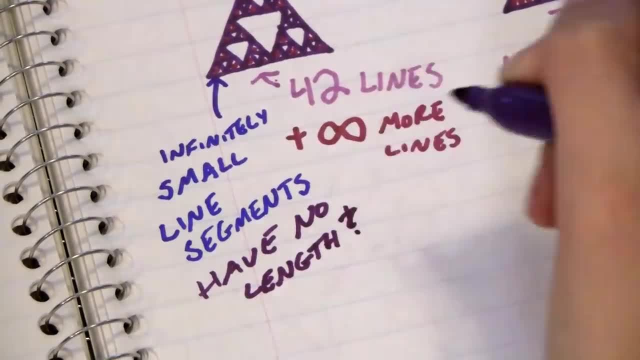 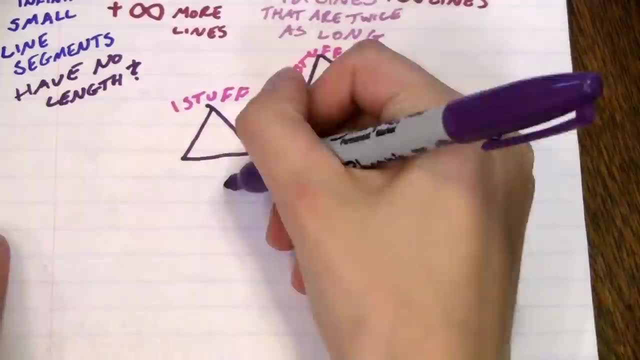 Wait lines that don't have length. Is that a thing? First, though, you figure out that when you make it twice as big, you get three times as much. Sierpinski triangle Not two like a 1D triangle outline, not four like a solid 2D triangle, but somewhere in. 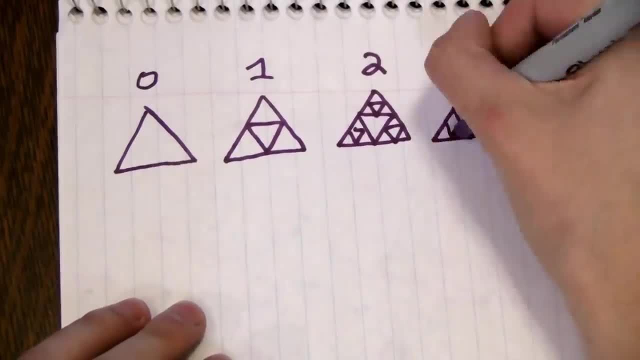 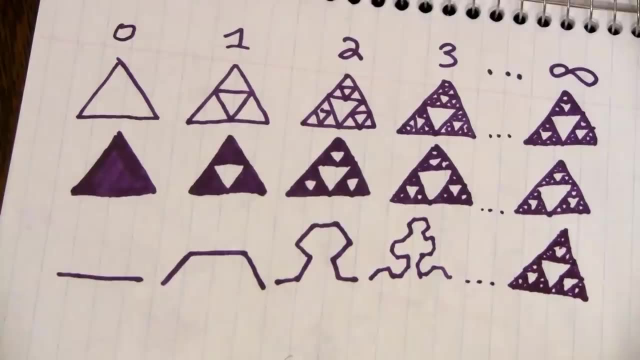 between And the in-between-ness seems to be true. no matter which way you make it out: of lines, or by subtracting 2D triangles, or with squiggles, they all end up the same: an object in fractional dimension, No longer 1D because of infinity, infinitely small lines, or no longer 2D because of subtracting. 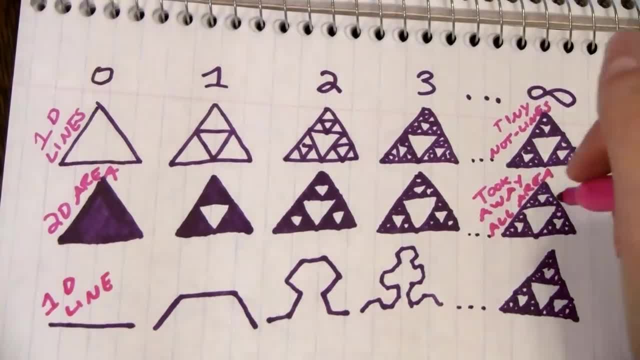 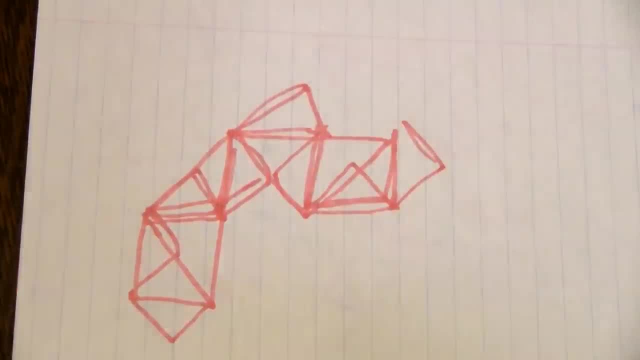 out all the area or being an infinitely squiggled up line. that's too infinite and squiggled to be a line anymore, but doesn't snuggle into itself enough to have any 2D area either, Though in the dragon curve it does seem to snuggle up into itself. 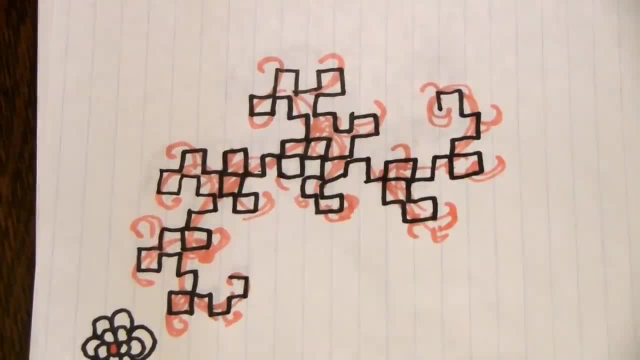 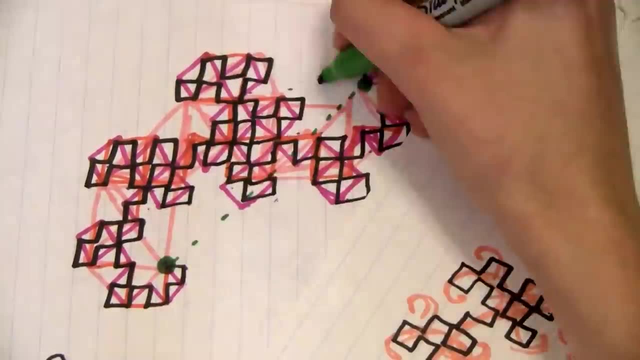 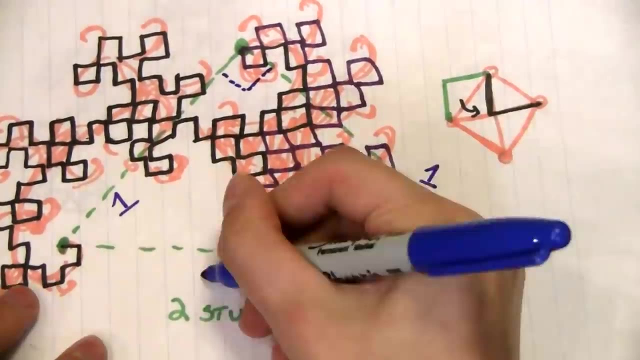 Hmm, If you pretend this is the complete dragon curve and iterate this way, there's twice as much stuff. that's what you'd expect from a 1D line if it were scaling up by two. But let's see, I suppose if you did it perfectly, it's supposed to be an equilateral right triangle, so square. 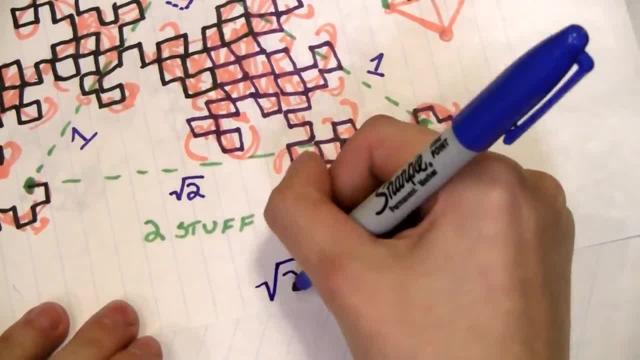 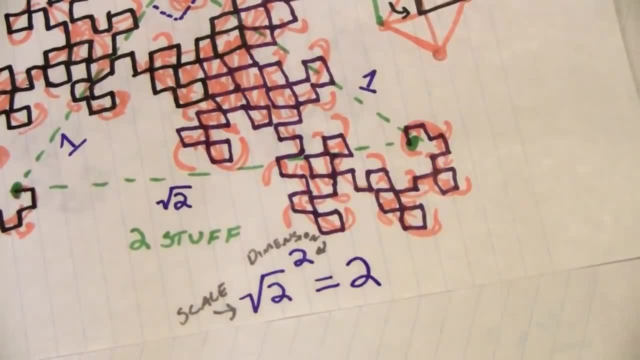 root two. Hmm, If it were two dimensional, you'd expect scaling up by square root two would give you square root two squared as much stuff. and square root two squared is of course two, Which is the amount of stuff you got. Odd how dragons turn out to be exactly two dimensional but in the end you get a filled. 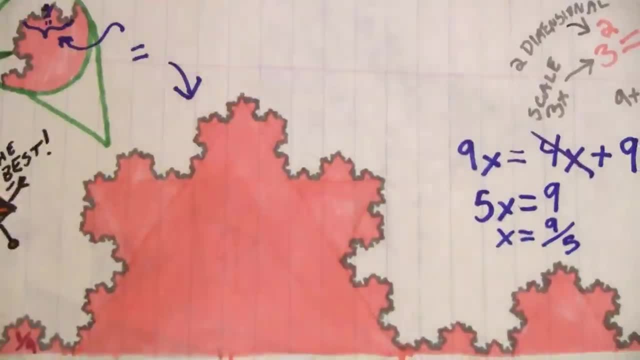 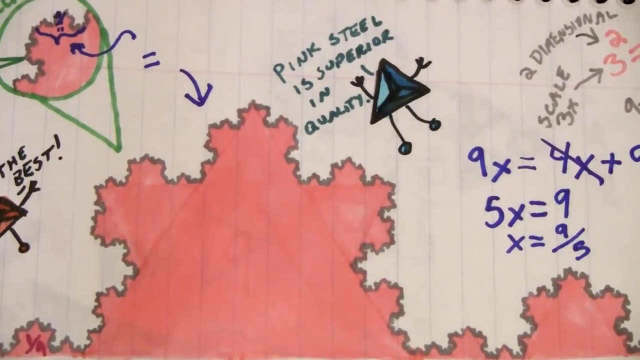 up thing with a fractal edge and that's a lot like a filled in dragon dungeon. 2D area of pink steel on the inside, Infinite fractal patina on the outside, Except the dragon curve still gets weirdness points for getting its 2D-ness from an infinitely. 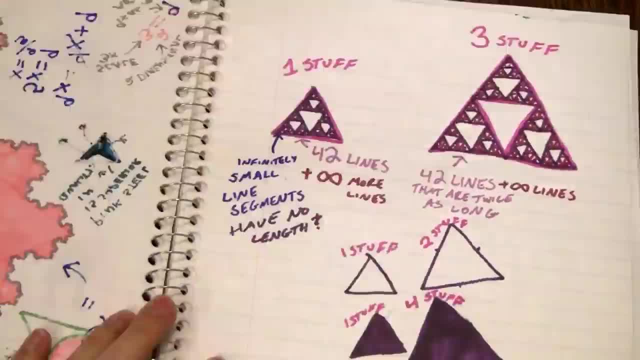 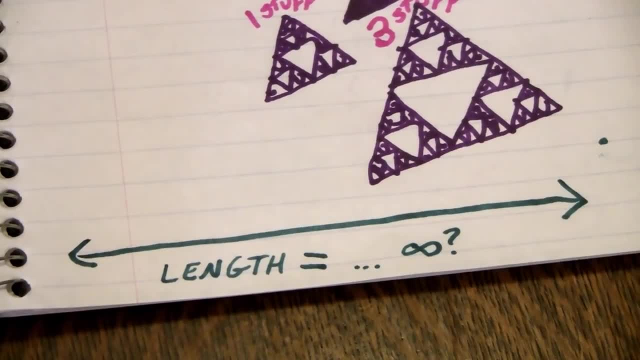 squiggled up line rather than triangles that are 2D to begin with. And now you're plagued by another thought: What about an infinitely long line, a true line, rather than the line segments you've been dealing with? In a way, an infinitely long line doesn't have a length, not a defined one. 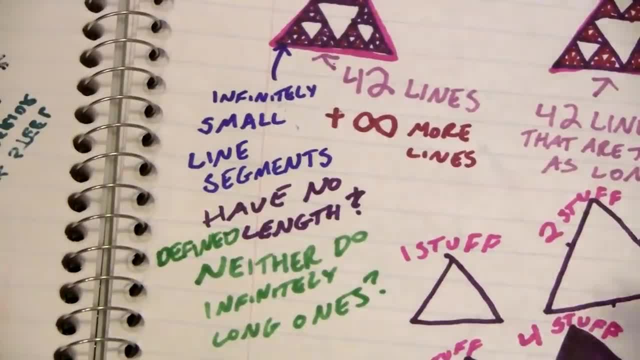 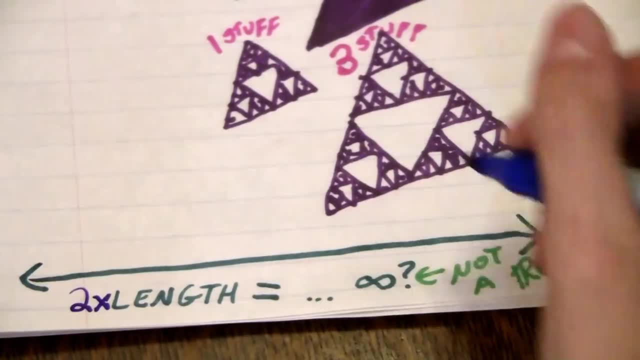 Like the infinitely short line, there's no real number capable of describing it. And if there's no number for it, How can you multiply that number by two If, when you make a line twice as long, you don't get a line with exactly twice the length? 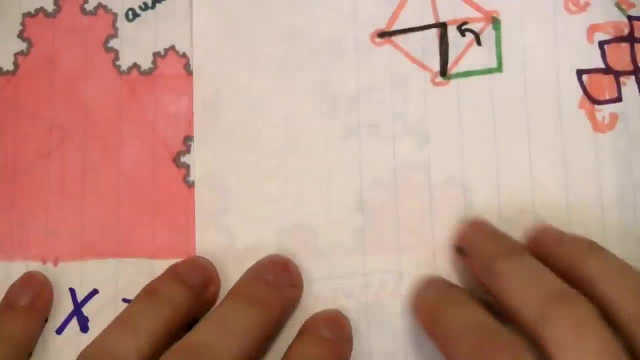 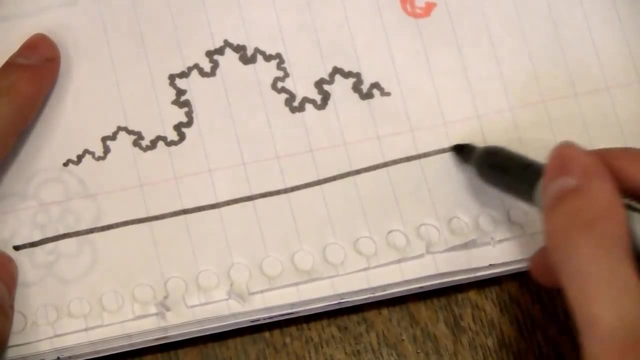 is a line really one dimensional? And if the Koch curve is made out of a line squiggled up enough to be more than 1D, what happens if you pull it back apart into a line? You try to imagine the correspondence. If this point ended up here, then this point would end up infinitely that way and this: 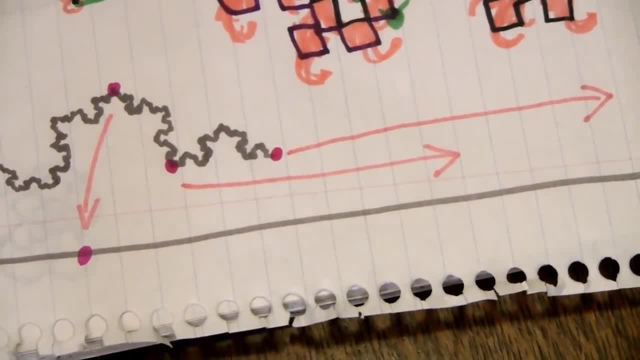 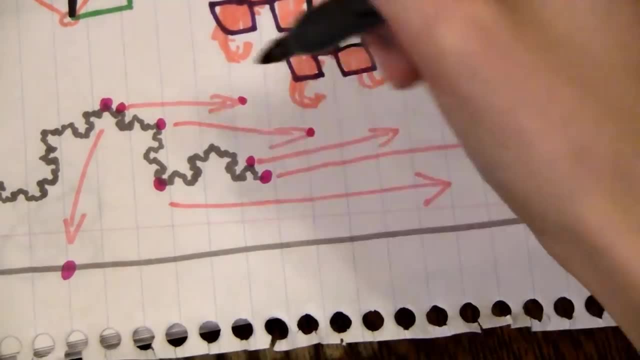 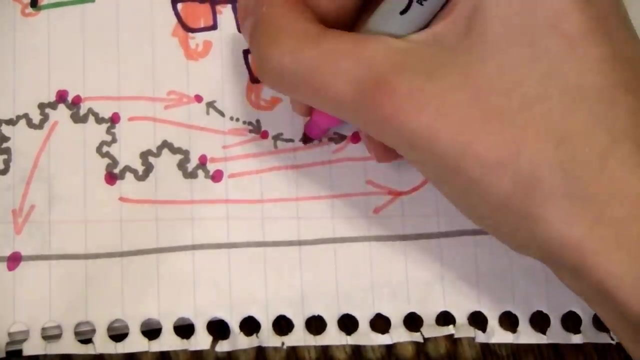 one twice as infinitely that way, which makes no sense, And this one also infinitely that way, and this one and this one, but they can't all end up at the same infinity because they each have to have infinite line between them. So you suppose you're going to need a super long line that's like infinitely, many, infinitely.